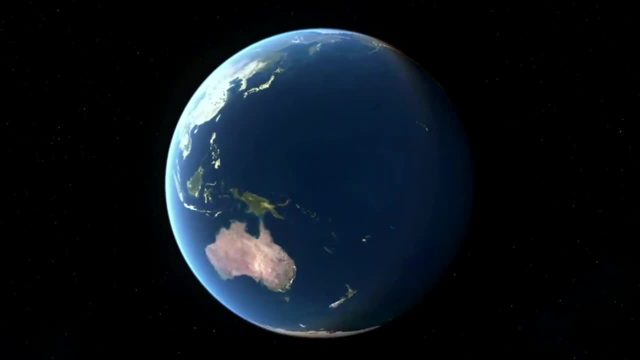 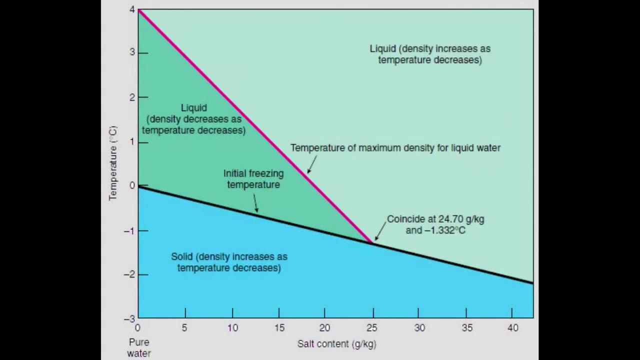 So let's talk about the main properties of these currents, how they formed and why. So it's the name effects of the water in the ocean. Very important ones will be the temperature, of course, and its salinity, so kind of like a composition of the water. 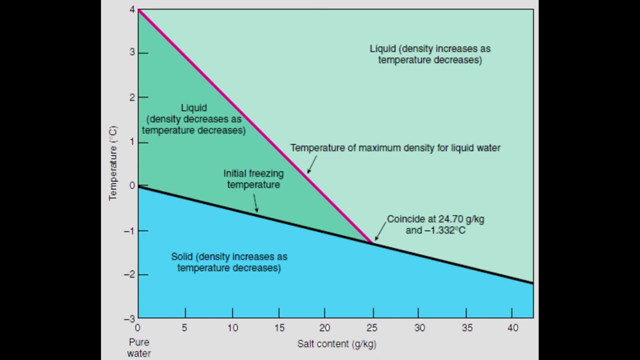 So the more salts you have in the water, the more denser it becomes. Denser it means it's become heavier, With similar effect. if you're cooling down the water or warming up the water, the density changes as well. In the studies of the ocean currents we call it thermohaline circulation. 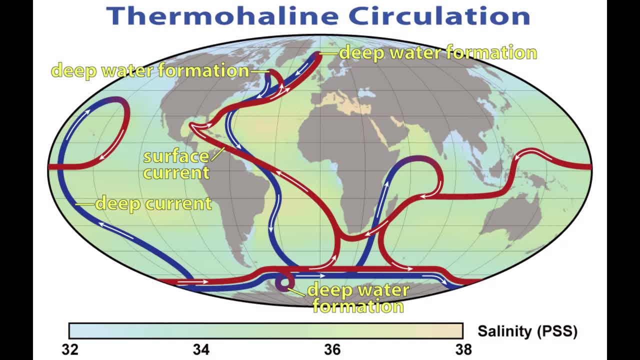 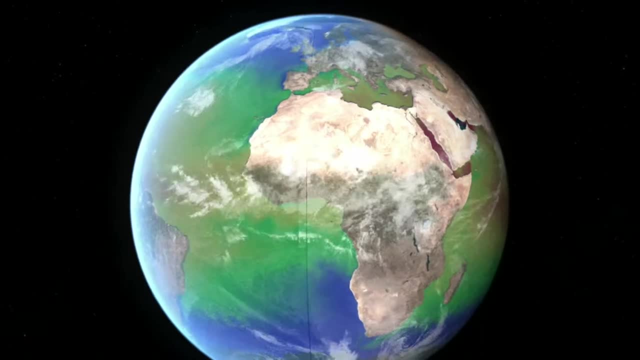 Haline means salt, thermo means temperature. So you have this effect of temperature and salinity affecting the ocean properties, and it's that drive the water to move. Another effect: you have cryolysis forces. Cryolysis forces: it's the force which act from rotation. 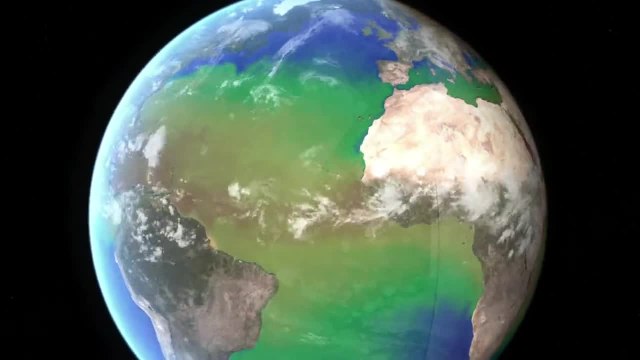 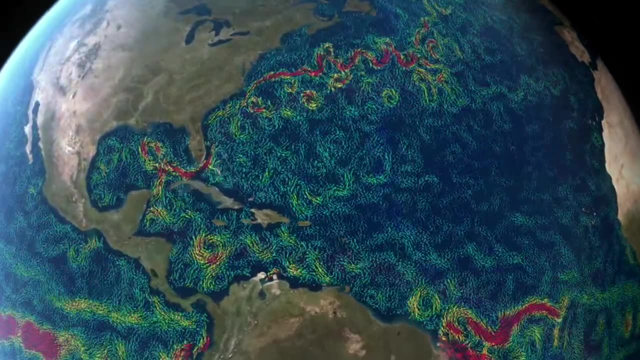 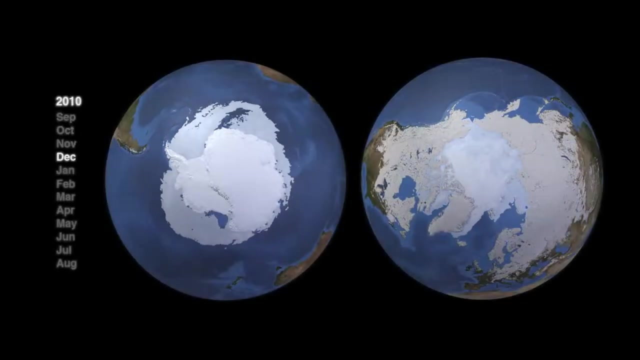 Cryolysis forces. it's the force which act from rotation And the rotation of the Earth around this axis. We have everything going a little bit clockwise in the northern hemisphere and anticlockwise in the southern hemisphere. You have the effect of the pressure in the atmosphere, precipitation, how much rain falls down and how much ice forms in the water. 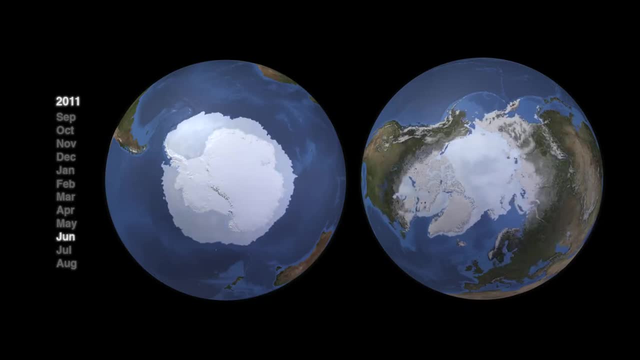 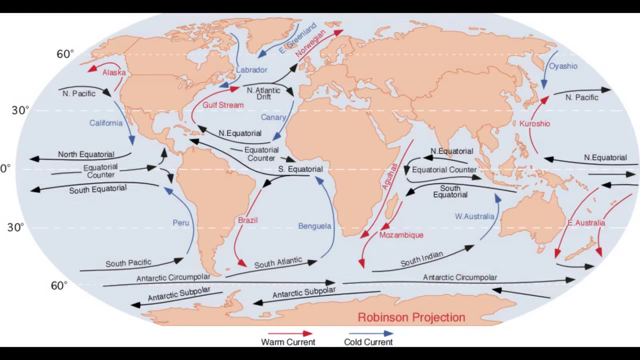 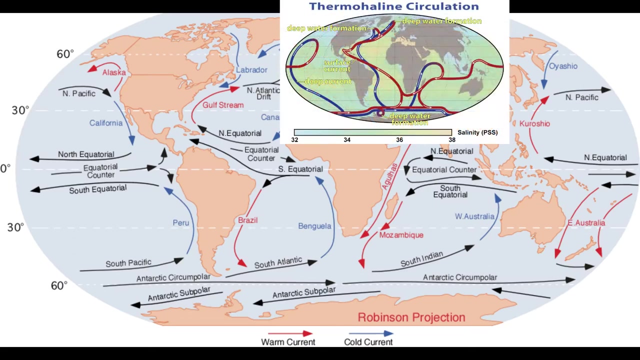 It will affect salinity and the density of the water again and will play a part in thermohaline circulation. So let's have a look on the Earth. On this map we see the main currents of the ocean. If you look it together with thermohaline circulation, one big conveyor belt of the mixing of the water and the ocean, they almost mix-match each other. 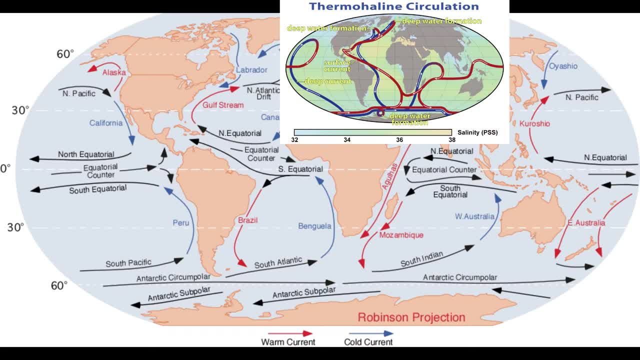 And we have particular patterns which preserve for many thousand years, with the current continent position and the bathymetry or the topography of the ocean which causing this movement of the water. When you think about the ocean, it warms up from the surface. 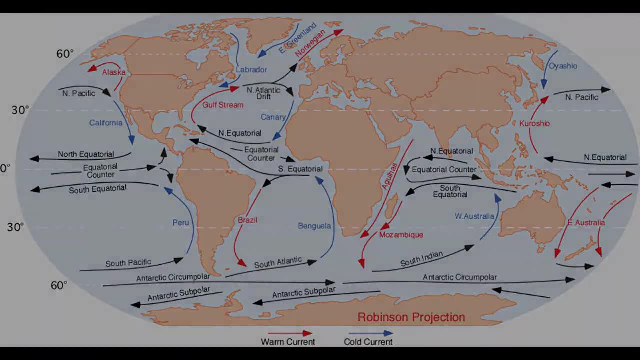 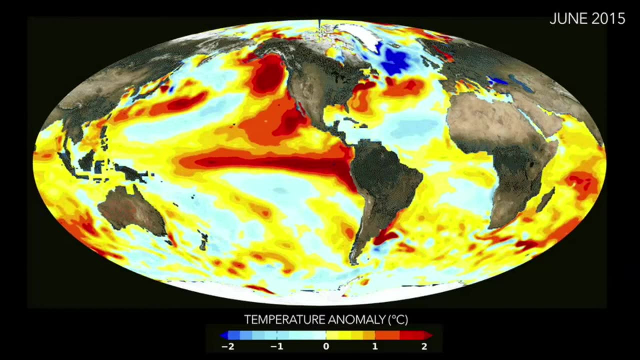 So we have warmer waters, heating up by the sea, Heating up by the sand And obviously, if I ask you this question, where will be the warmer waters? you will tell me: around equator, And it's absolutely true. Around equator, in tropical areas, we have the warmest waters in the ocean. 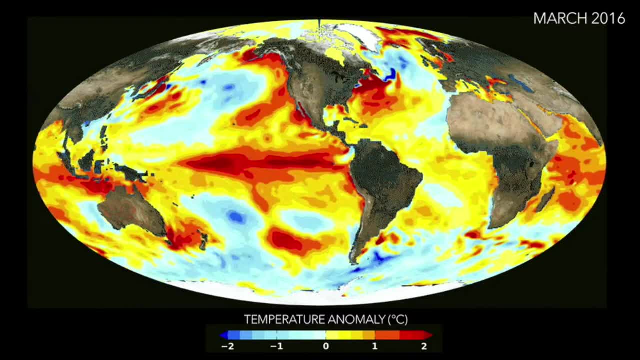 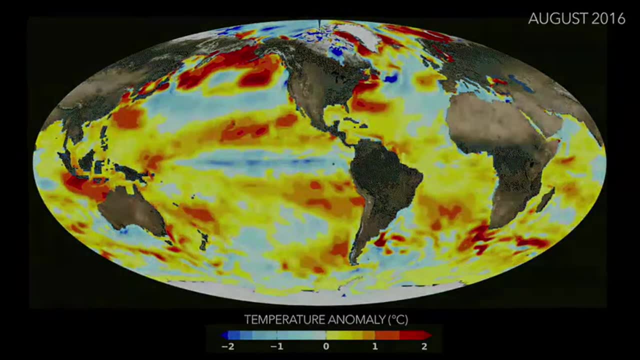 This water warms up A lot of rain falling down in tropical area. It changes salinity, Make it a little bit fresher And, as a result, water start move. Obviously warmer water start move towards northern pole and towards Antarctica, southern pole. 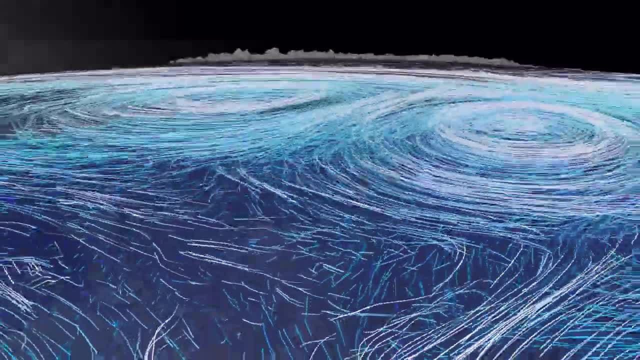 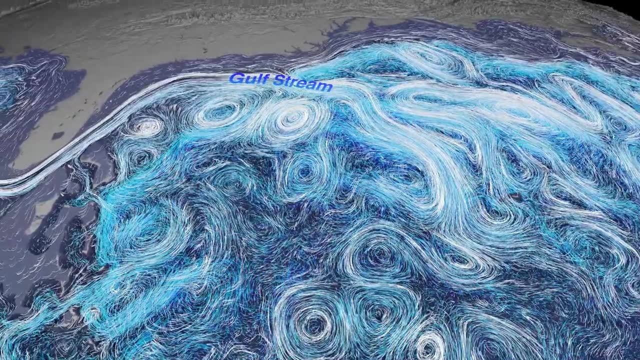 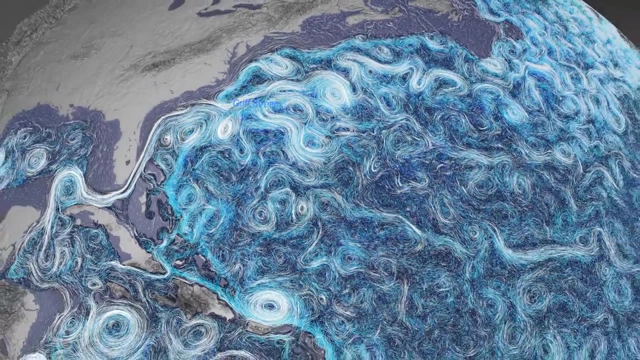 But the temperature changes. It changes As the climate moves. it will be a little bit directed by exposition of the continents. If you look in the Atlantic Ocean, we have the big current coming towards Central America, Heating off the east coast of south of Northern America and then moves through Atlantic towards Northern Europe. 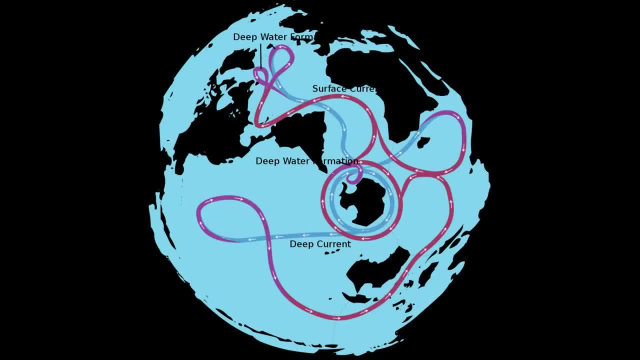 We call it Gulf Stream. In the thermohaline circulation, it's the main current of the warmer waters, Then going up all the way till the Northern Atlantic. On the way it brings warmer temperatures and more rain to the ocean- Rain to the Europe. 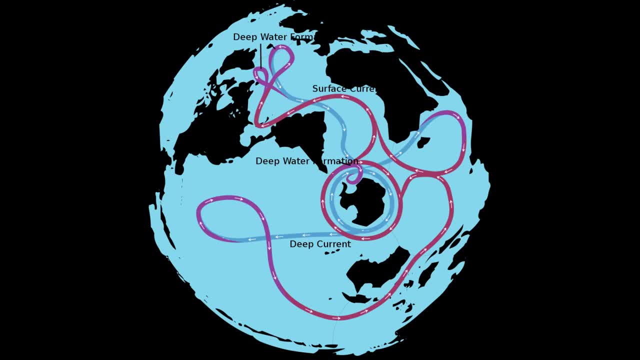 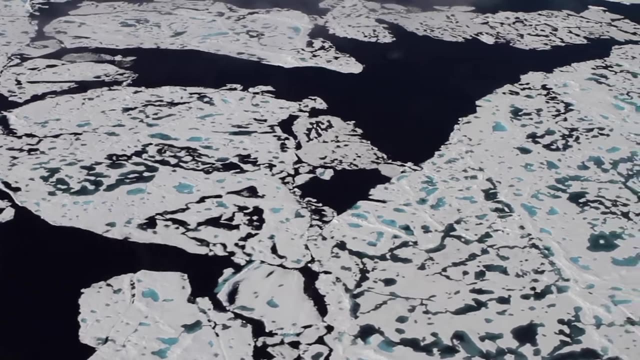 Make it climate more temperate and warmer than climates on the similar latitudes in other places. When it reach the cold northern regions, the water cools down On the way. it's become already not as hot. The ice start forming in the winter seasons, which increase salinity of the water. 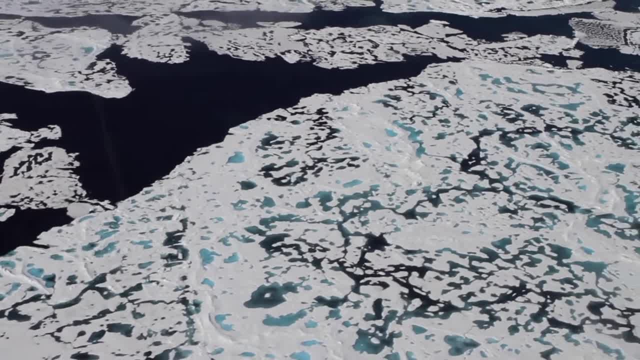 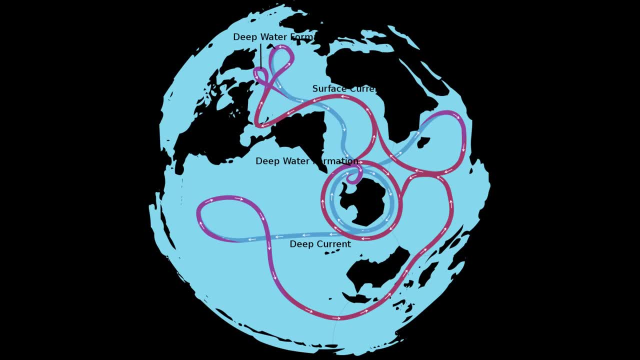 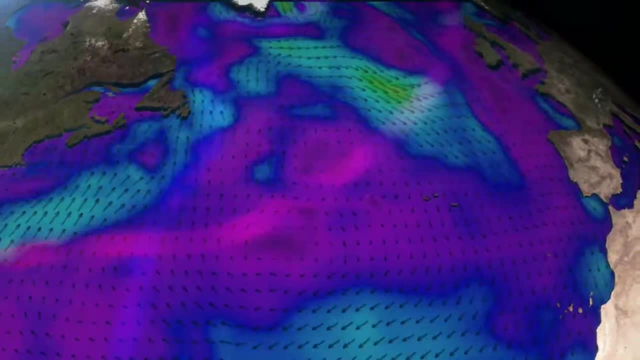 Because when you form the ice, the salt not become part of the ice. It's left on the surface of the ocean And, as a result, Colder and more salty Waters become denser and they sunk down towards the bottom. These thick layers of the colder, denser water start moving back south. 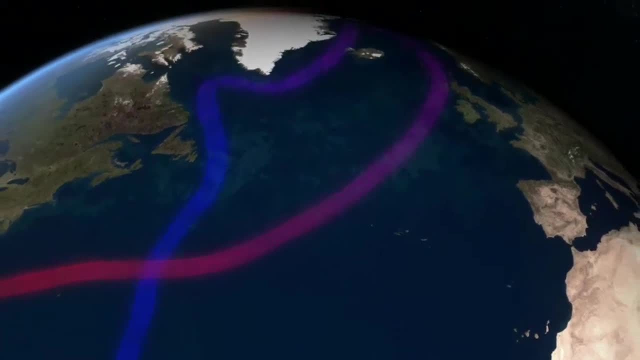 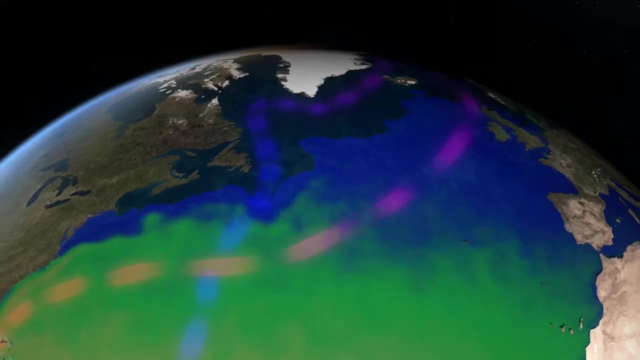 It's compensate for those waters that move from south towards the north, The warmer waters we talked about, And it's gonna compensate. So we have this undercurrent underneath of the ocean, at the bottom, Which go in the opposite direction of the warmer Gulf Stream. 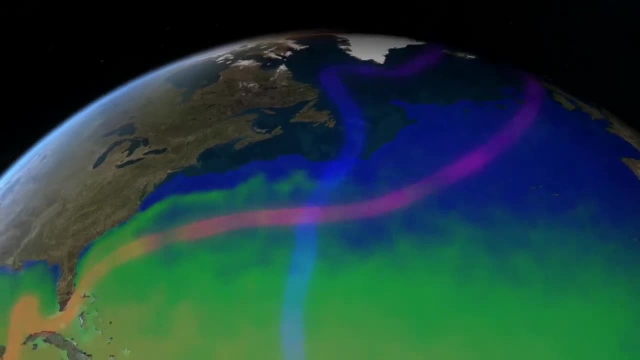 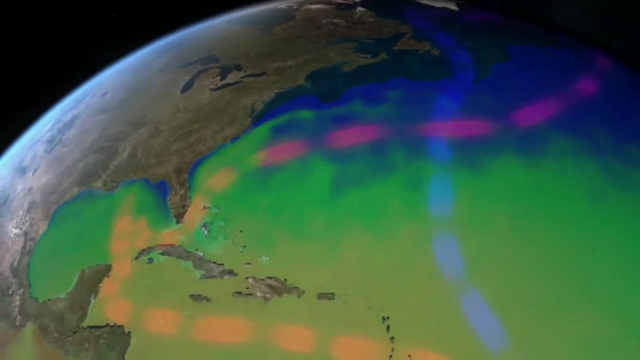 Warmer stream going north As a result, All these colder waters going all the way down Until equator. On the way it will start slightly warming up, But because it's located in the bottom of the ocean It'll be very hard to warming up through. 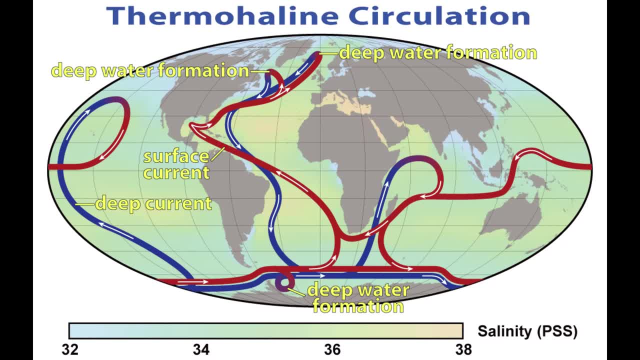 Can imagine, to warm up through 3,, 4,, 5 thousand meters of water. You have this warmer current and surface And you have colder waters underneath. Usually they not mix very well there. These colder waters reach till Antarctica And then they join all these circumference big current around Antarctica continent. 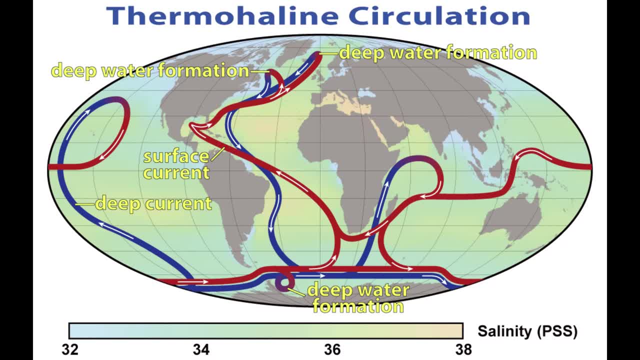 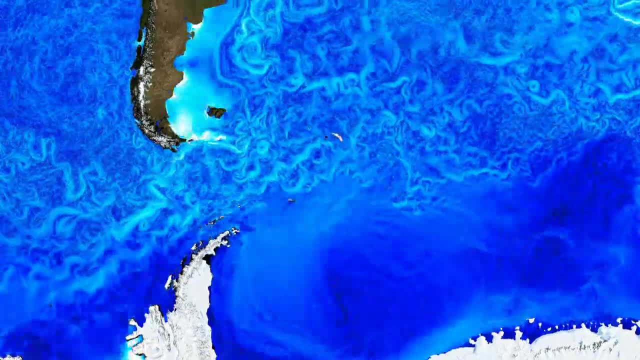 You can see on the map, It's the biggest big current Which move eastward all around Antarctica. Then some of the waters will branch off Towards the Indian Ocean and Pacific Ocean, Where it'll be entrained by this replacements of the water waters. 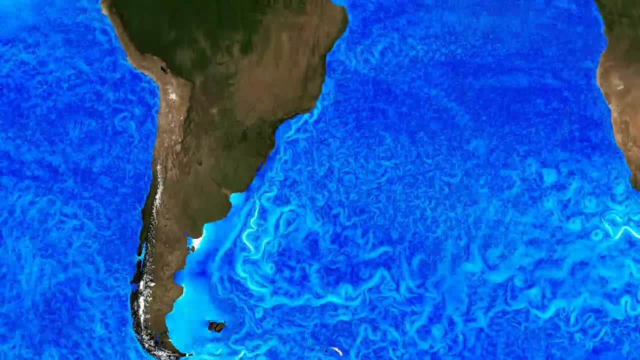 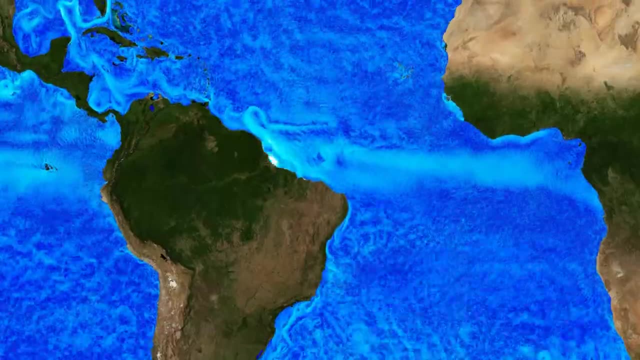 Which constantly going away from the equator And will be driven up towards the equator In the places where colder water will come towards the surface- We call them upwelling areas- We'll have the transition of this colder, denser bottom layers. 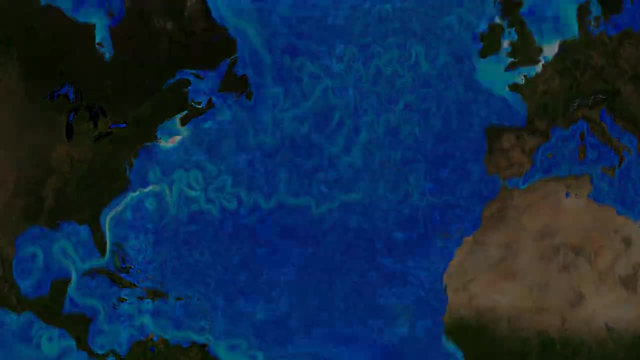 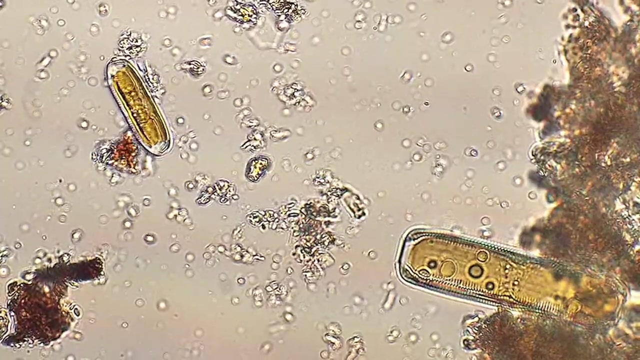 Into the surface warmer layers of the water. You can see on the map where this happening And usually you know these places by very rich ocean life, For example. a lot of nutrition be brought with the colder waters. Plankton will love that area. 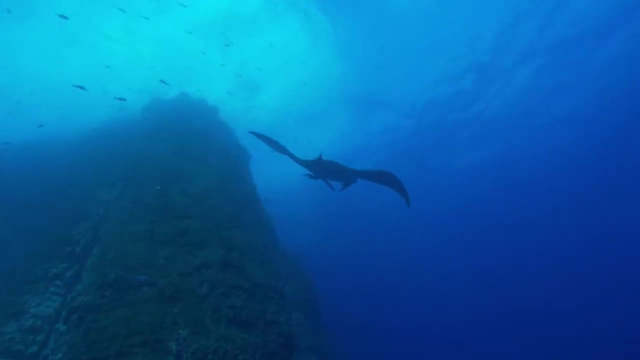 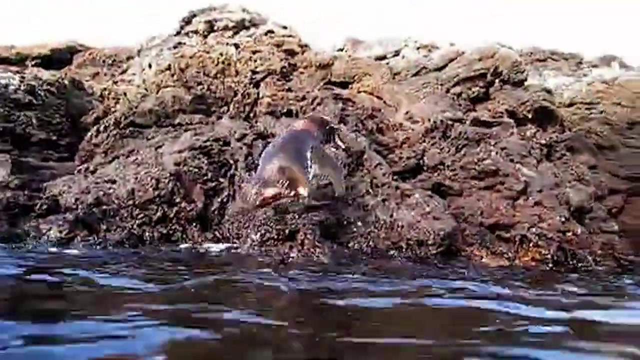 So there'll be a lot of plankton, And where there's a lot of plankton, There'll be numerous lives, Fishes, mammals and birds. If you're a fisherman, you know there's areas, Because that's the places where people fishing mostly. 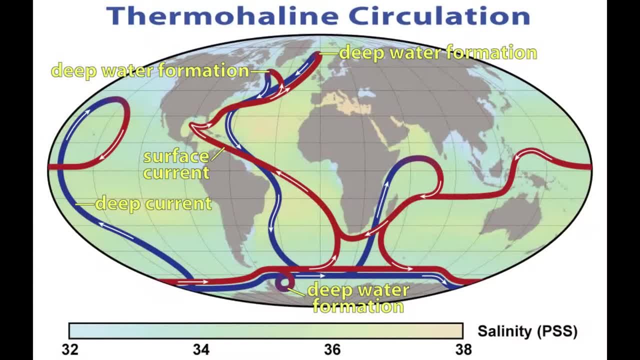 Then this warmer waters will become on surface of the colder layers And it will continue the circle back down From equator warmer areas towards the poles. If you look in the map of thermohaline circulation, This is the main conveyor belt. 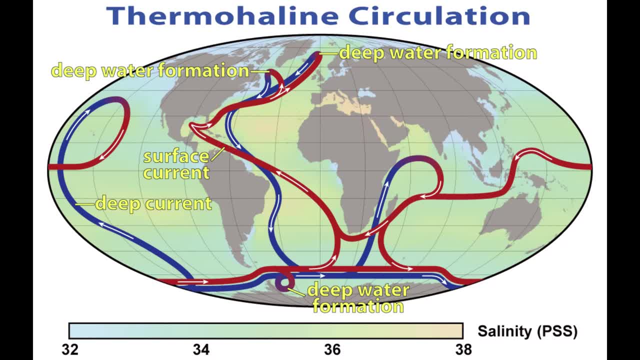 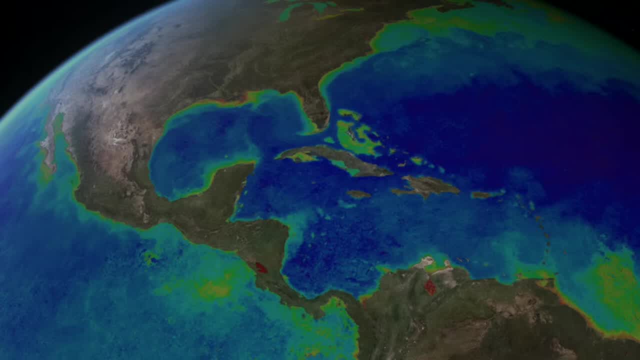 It's moving through the cycle of the waters. It might take about one half thousand years For water to travel through all of the oceans And finish the cycle. Therefore, although it seems like our oceans are separate On the surface of the planet, 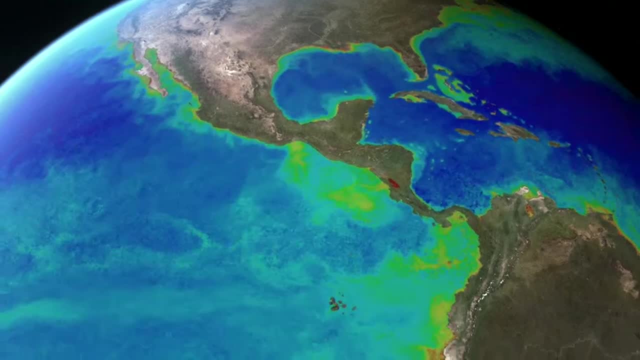 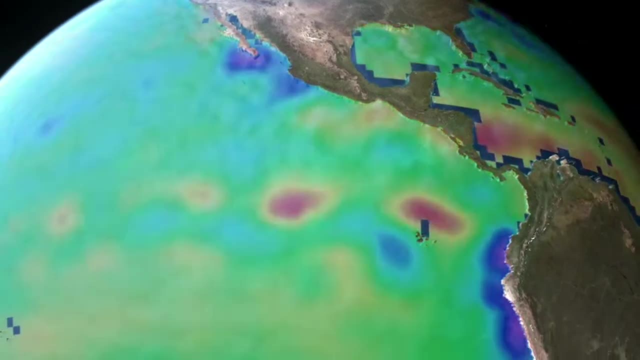 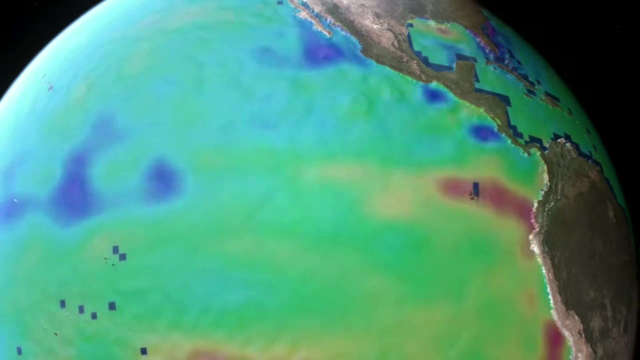 Four main oceans. They do mix, But just slowly and gradually with time. So the ocean body around the planet work as a cooling mechanism. So it's constantly moving the warmer waters from the equator towards the north. In the same time it's also preserve the heat that collected. 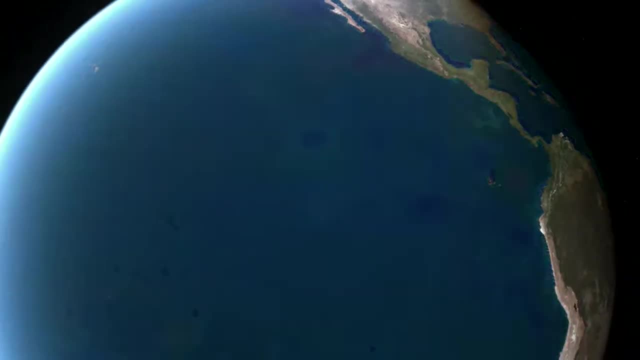 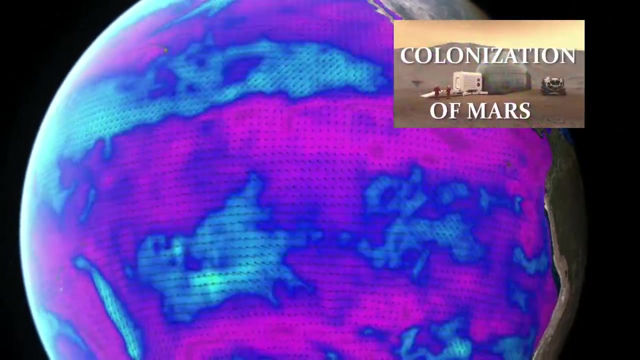 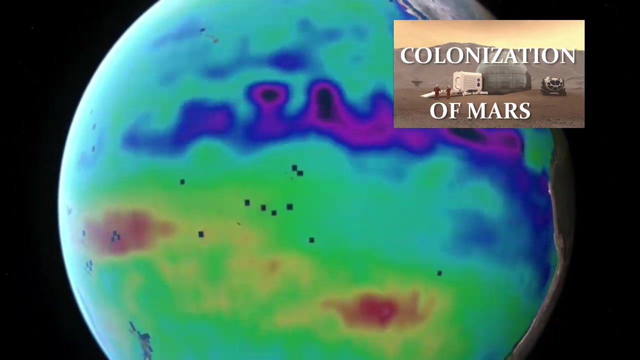 Through the seasons by the ocean And then very slowly release it, Making our temperature on the planet surface more temperate, Which my other videos about Mars and Mars And Moon, Where we talked about how just the land Much faster heat up through the warmer periods. 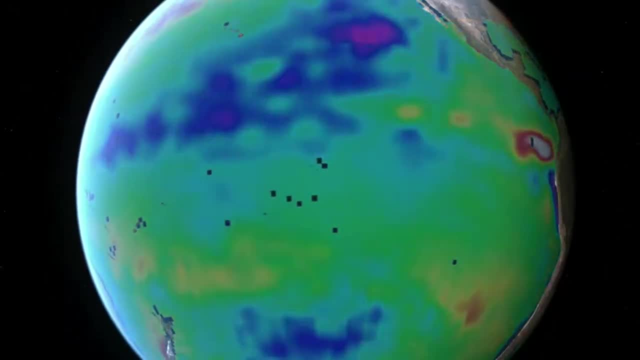 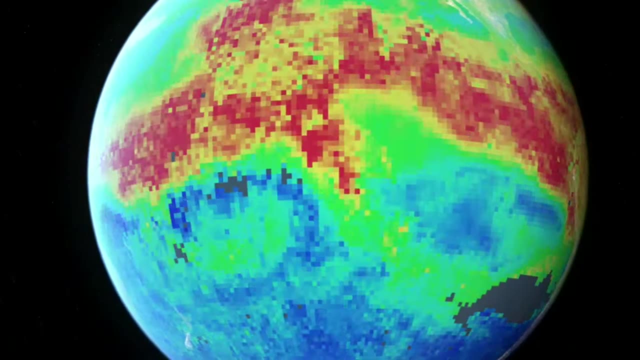 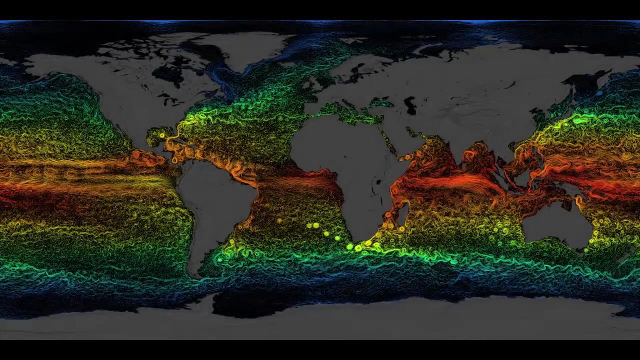 And release the heat very fast due to the density Water, as a result, work as a cover for our planet, As the atmosphere as well, Which effectively redistribute the heat throughout And for us, for people, It works as a natural heaters And if you look on the ocean current map: 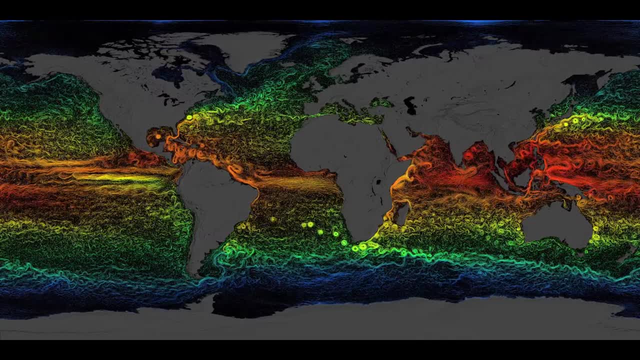 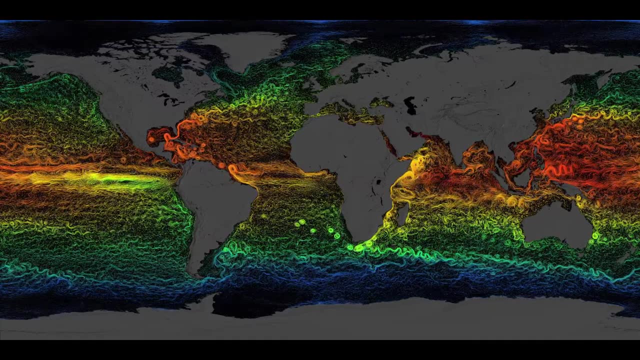 After you understand thermohaline circulation, The main conveyor belt of the ocean waters in a global ocean, You see that it's related to that. But we just have some local branches out When smaller currents coming out from the main thermohaline currents. 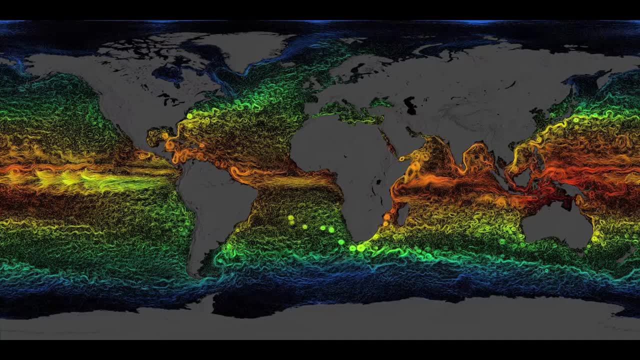 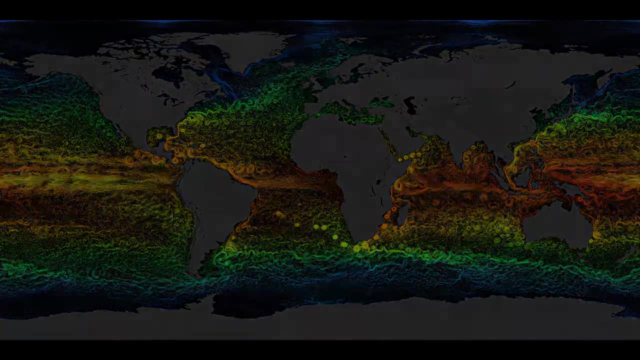 And they will affect locally the climate of particular areas of the planet. For example, Gold stream, The biggest and the most famous warm current of the water in the northern Atlantic. It's related to thermohaline warmer current coming all the way up. From south Atlantic till the north And you have some compensation currents going in opposite directions With opposite temperature. You have to. If you bring the big current of the warmer water in one place, The cold water will have to leave that place. Some currents will be shifting north-wise or south-wise. 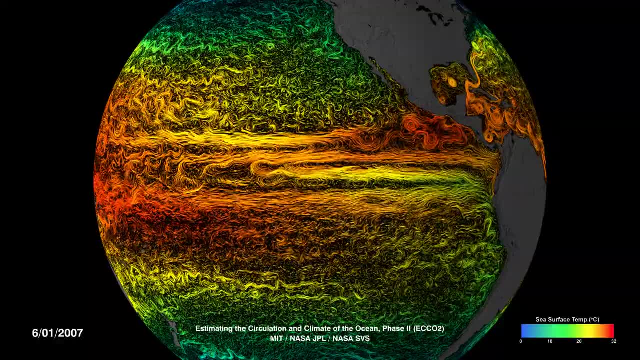 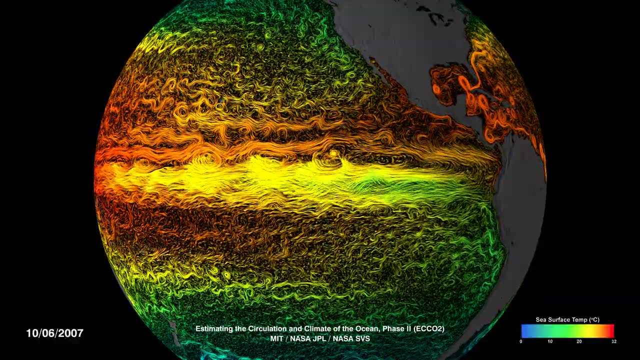 Depending on the seasons, And they become less strong or more prominent as well. However, they stay like that for some time. We know through that. We know through the climate studies, Paleoclimatology, That some currents been there for long time. For thousands of years with us. However, For example, During the last quaternary period, Glaciations affected some of the currents. When you have increase of glaciers on the planet, Less water become in the ocean. Some lands get exposed. 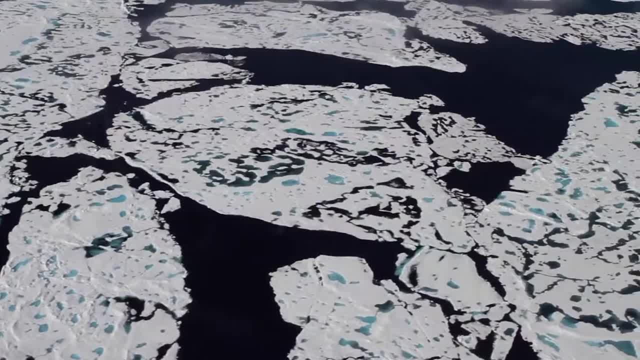 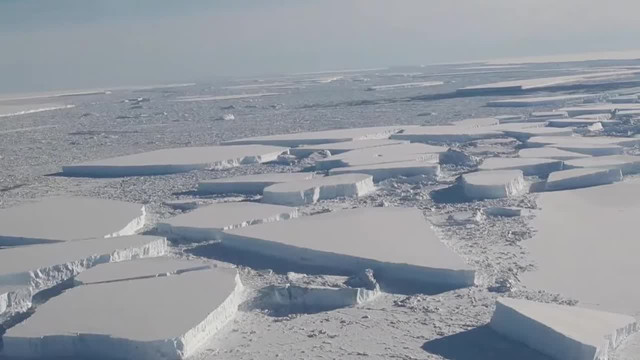 Costs. Ocean become saltier Because of all fresh water trapped in the ice. You will have particular patterns Of the ocean circulation When you start melting rapidly All those glaciers, Big flux of the fresh water Coming from the continents Down into the ocean. 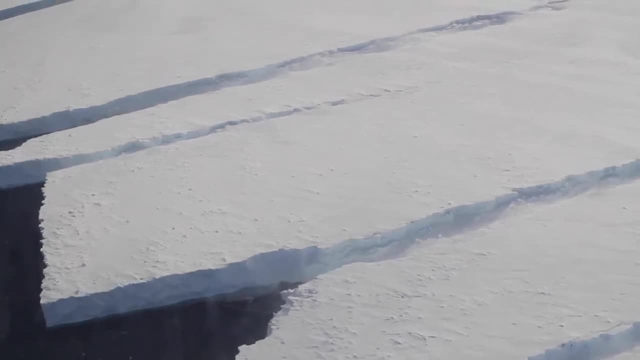 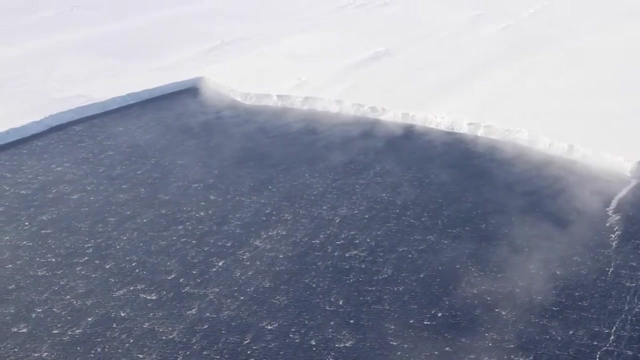 The fresh water from the continents, Coming from the glaciers, Will not straight away mix With denser, salty water of the ocean Which already underneath And as a result, There will be some readjustments happening Which paleoclimatologists studying. 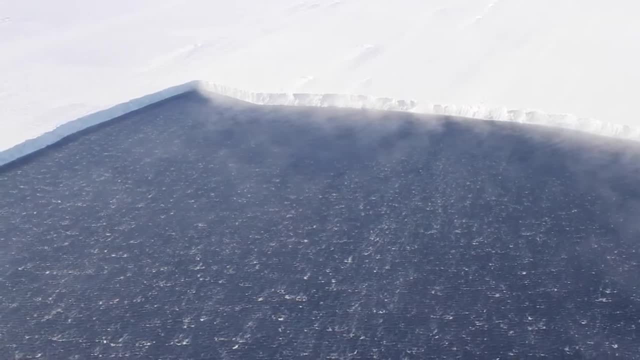 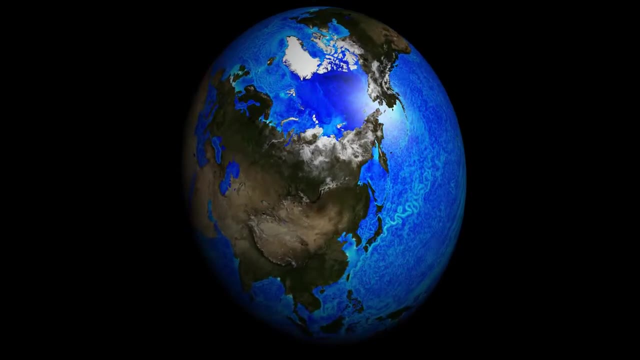 And eventually the ocean currents will restabilize, Find new patterns And we see the modern picture of the currents. Therefore, you can see That the global ocean patterns Will affect the local climates For the land, Bringing warmer air Or colder air. 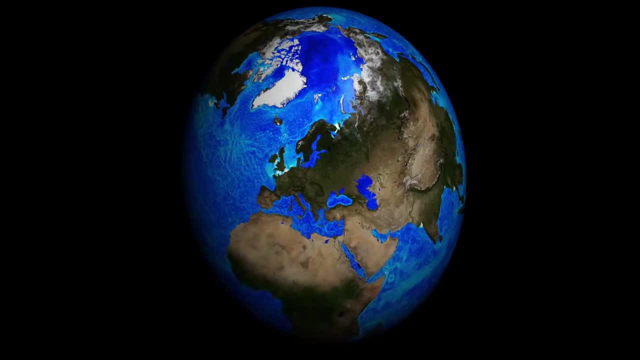 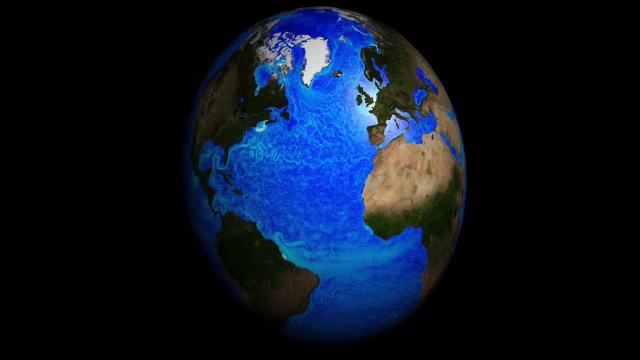 For example, As we already mentioned, Western Europe and England In particular, warmer places In comparison with North America, Same latitude Because of the warm effect of the cold stream, We have more rain, Warmer air coming from the ocean And dominated western winds.